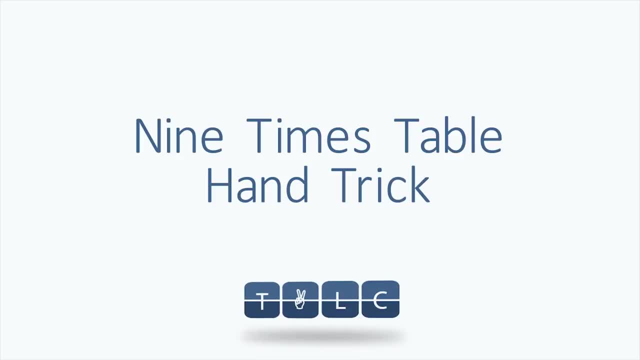 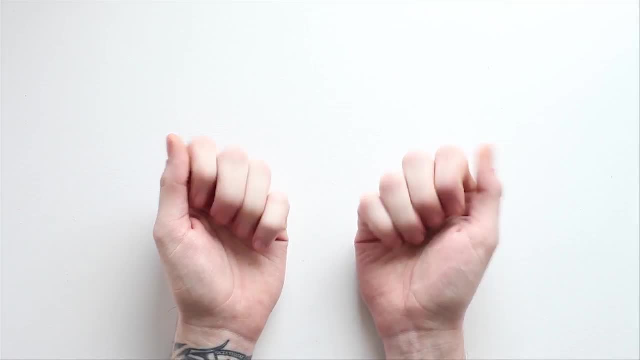 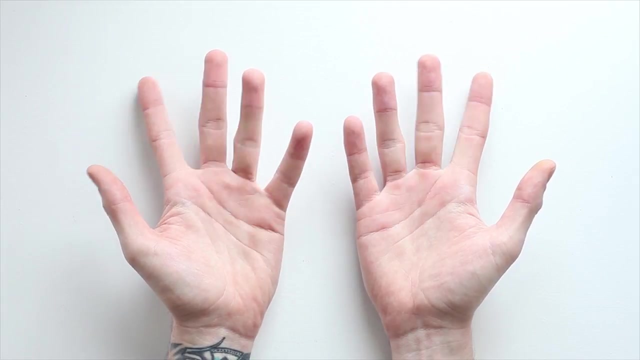 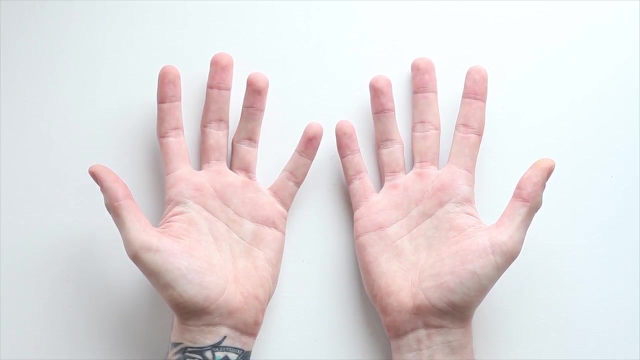 Hold out your hands in front of you so you can see your palms To show our nine times table. we're going to use all ten fingers. There's a pattern, see, And we can show it. if we fold down one finger or thumb at a time, Starting with your left thumb, we can now number all your fingers up to ten One. 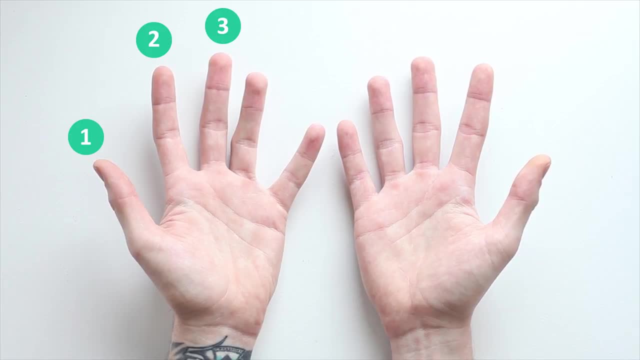 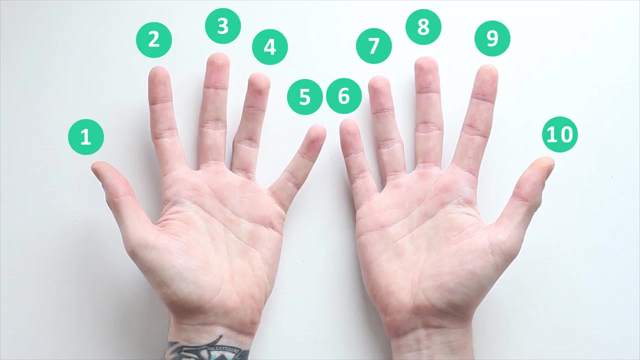 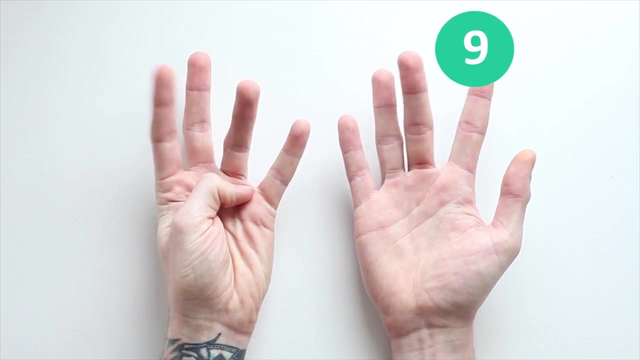 two, three, four, five, six, seven, eight, nine, ten. Now if we want to know what one times nine is, we start with that left thumb. Fold it down close into your hand, Then you can see nine fingers still standing. So one times nine is nine. Okay, 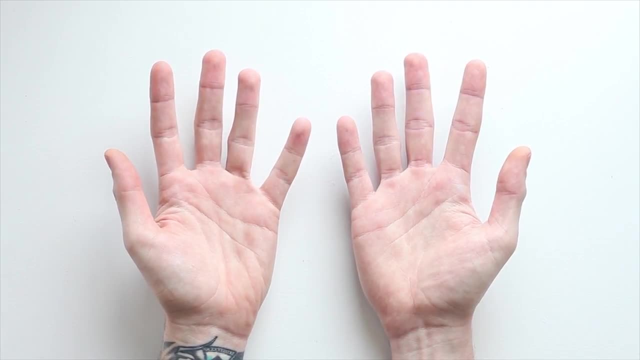 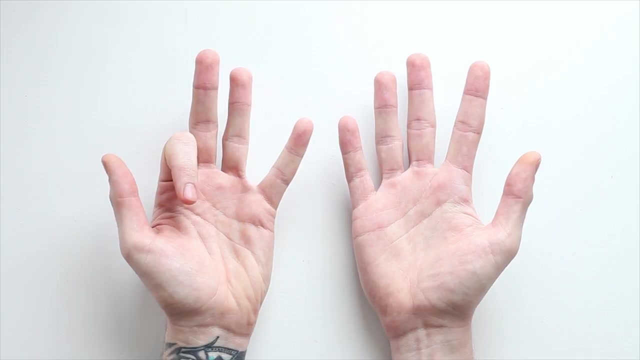 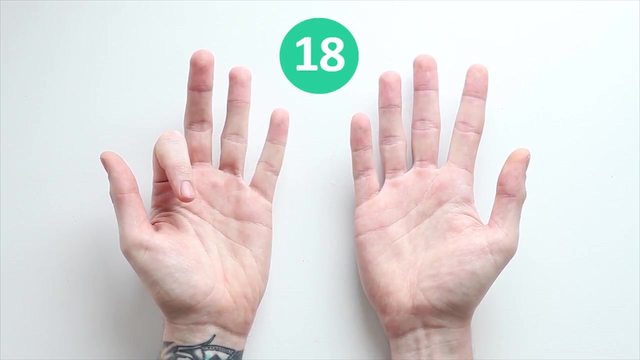 put your thumb back up. Now we can do two times nine This time. fold down your first finger, the one we called two. On the left of that finger is one thumb and on the right are eight other fingers. One and eight, that's eighteen. So two times nine is eighteen. In maths we often talk. 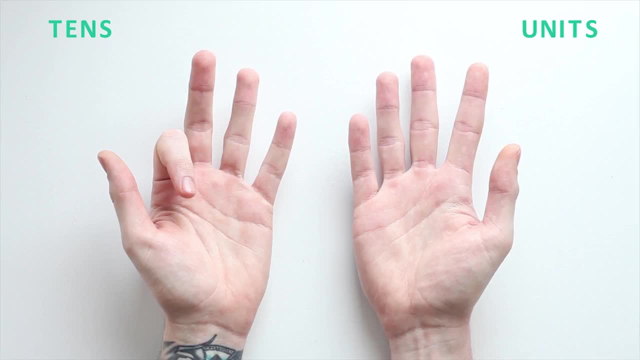 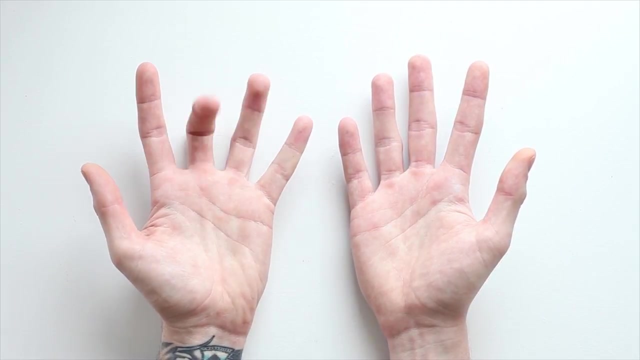 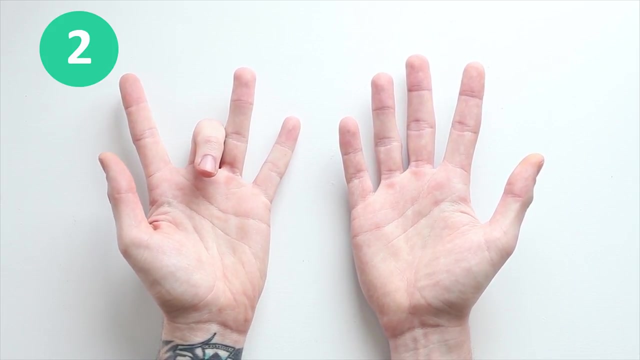 about numbers being in the units column or the tens column. and that is what is going on here. Tens on the left of your folded finger, units on the right. Try the same again with three times nine Fold down. the middle finger, number three. Left of it are two fingers, Right of it are seven fingers. 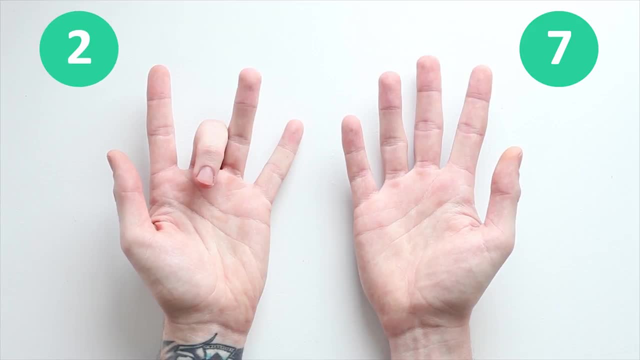 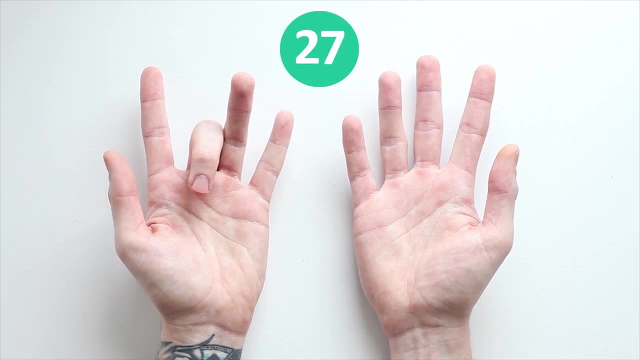 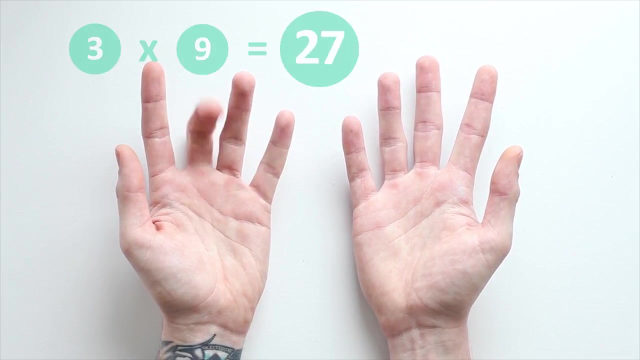 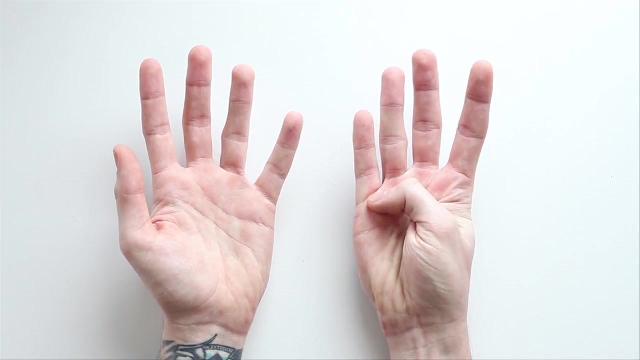 Two tens and seven units. Twenty and seven, Twenty seven, Three nines is twenty seven. This works all the way up to ten times nine. By the time you get to the thumb on your right, you will have reached ten times nine.